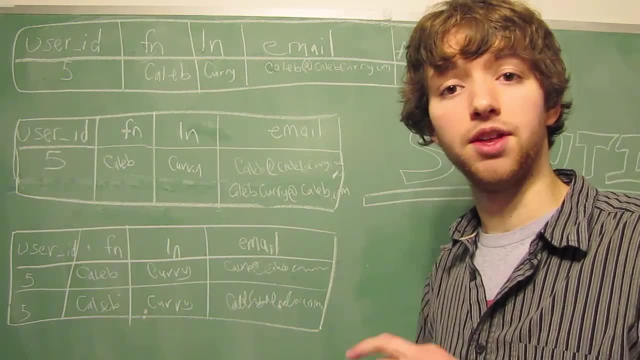 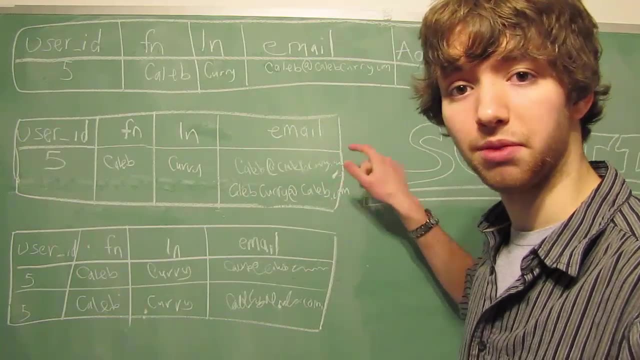 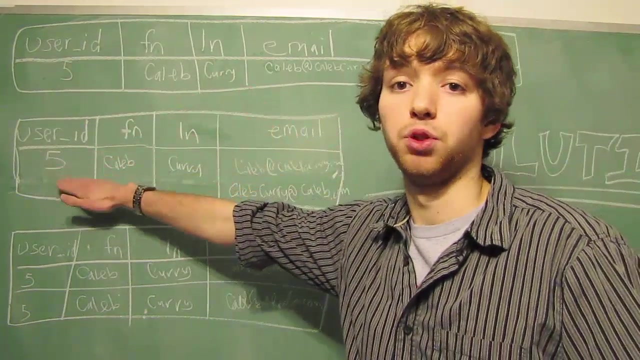 email. Imagine putting one email in and then putting your second email in in the same box and clicking submit. Well, it's entered into the database as a single value, maybe with a comma or something, but it's still entered in as the email for this user. So two values within one, which? 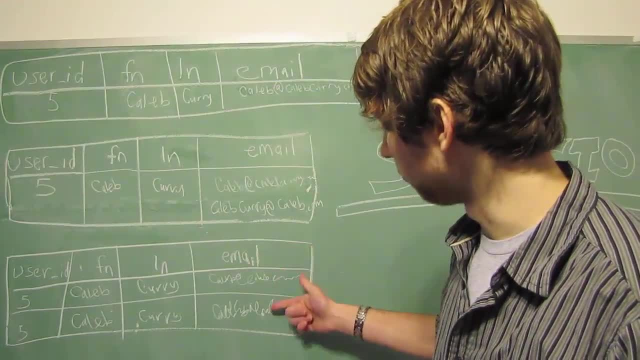 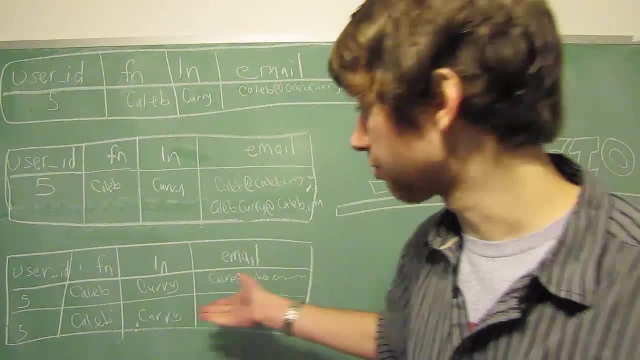 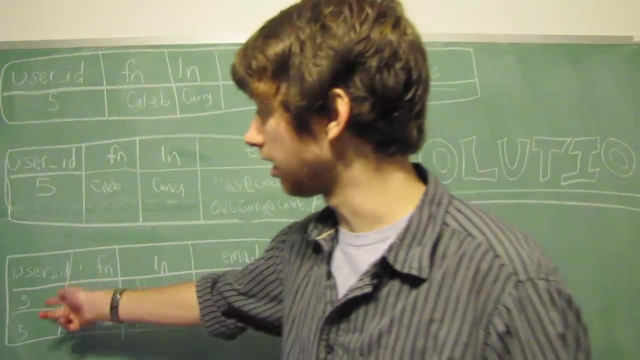 is not atomic. In this example, the actual values given for the email are atomic because they're only one email, but we put two entries within our database. So now we have this in here twice, this in here twice, And the primary key should never be in there twice, The only time you can see the primary. 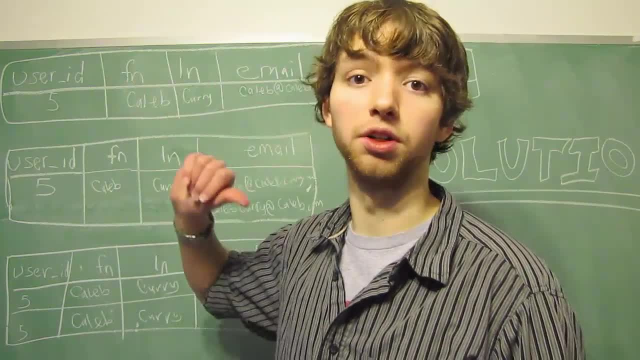 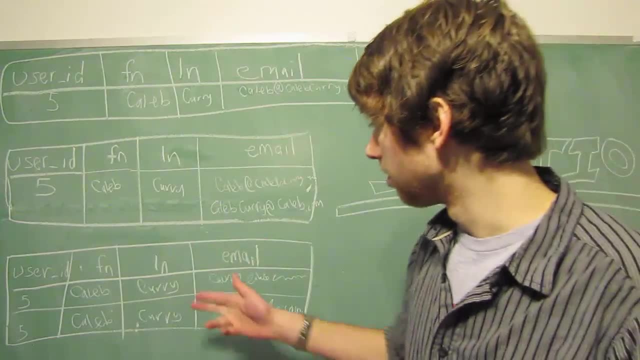 key in there twice is if it's a reference as a foreign key, because a foreign key can be put in there multiple times, But the primary key of five should only be in there one time. So we have all that duplicate data. Now what if this Caleb Curry goes and gets a name change, Because that's such a dumb. 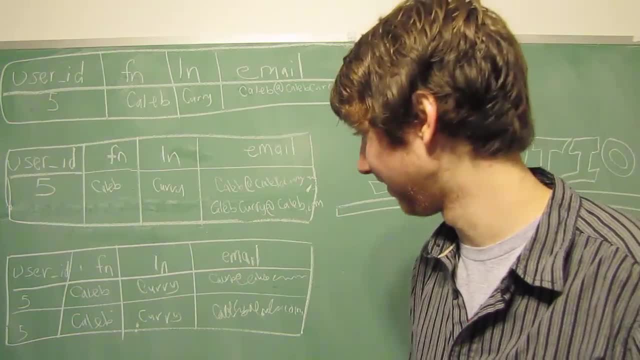 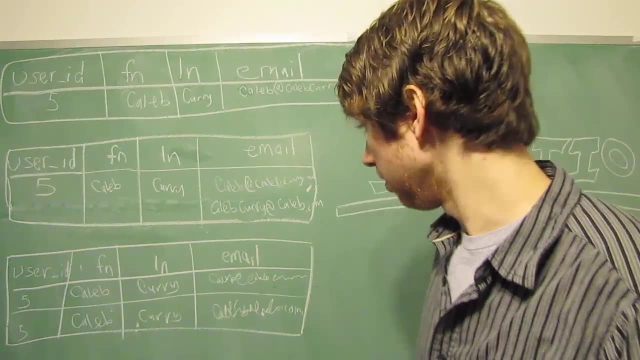 name right? No, I'm just kidding because that's my name And I actually like that name. If he gets a name change and he updates his information, what if only this one's updated? So now we have conflicting data And see, that's the problem with data integrity. We 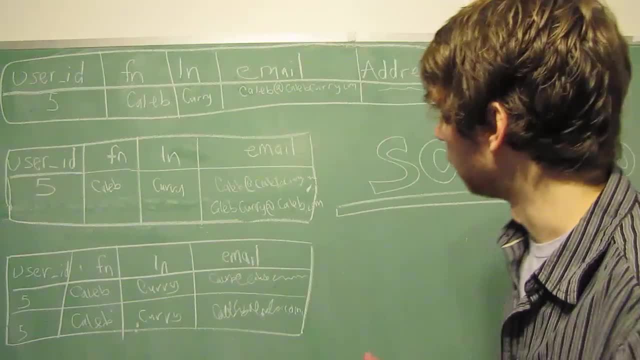 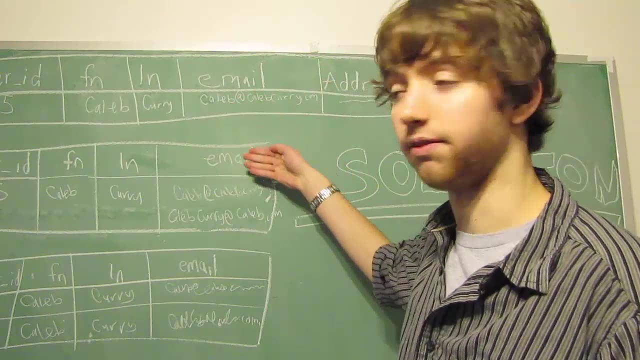 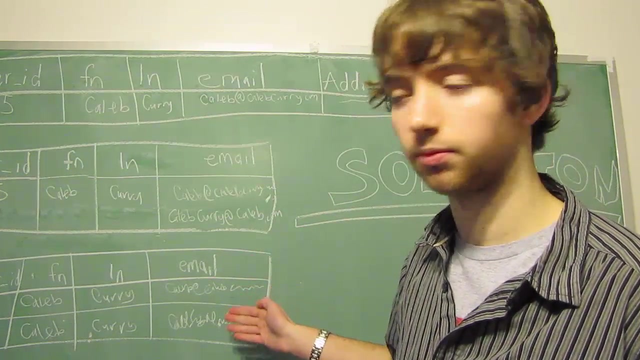 need to make sure that doesn't happen. So in this example, the column is the problem, In this example, the values for the row is the problem, And in this example, the values for the row is the problem. So these basically have the same problem. 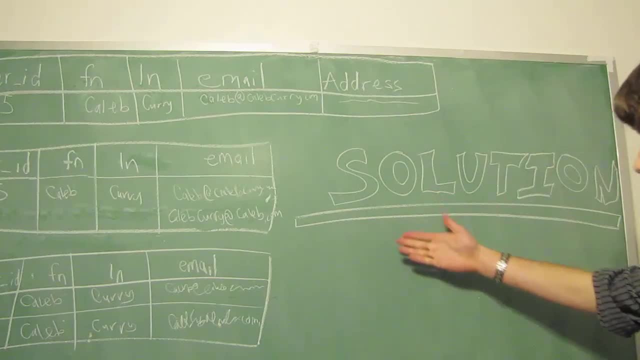 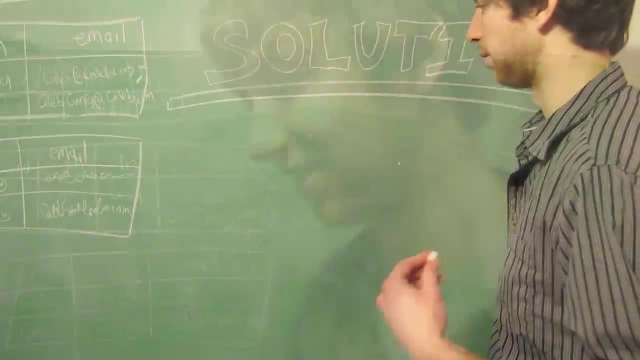 How do we figure out the solution? Let's take a look over here And, as you can see, there is no solution. So yeah, guys, thanks for watching. I'm just kidding. Let's do this. The best solution for this problem is to have a user table, And I'm going to write the columns that are: 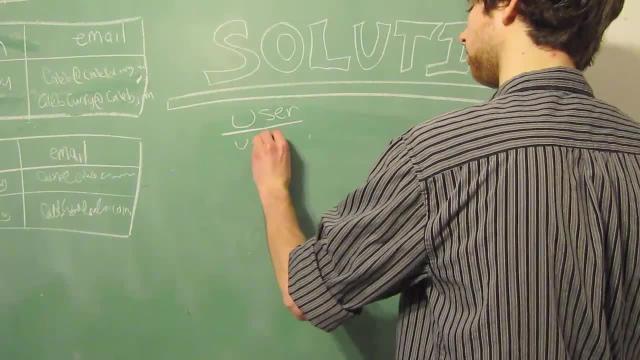 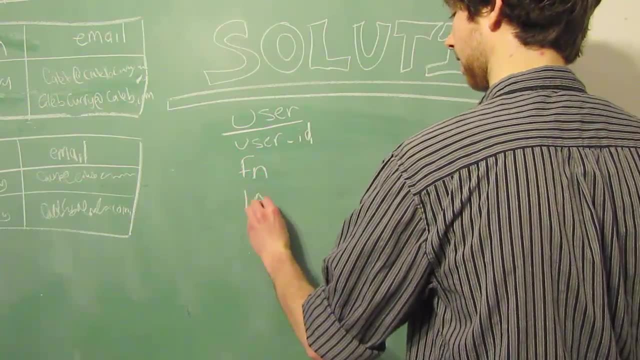 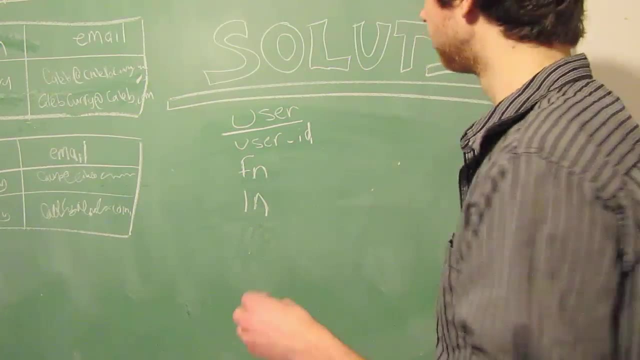 within this user table, So we would have a user ID. Then we are going to have a first name And we're going to have a last name. If you wanted the address in there, you could have a street address, state, country, all that other good stuff. 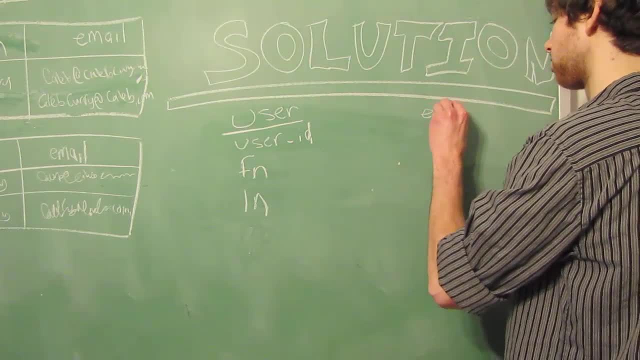 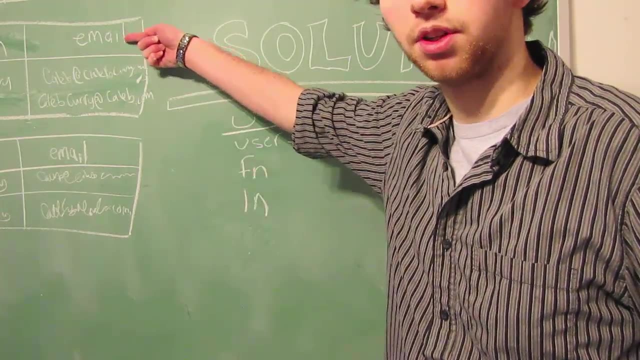 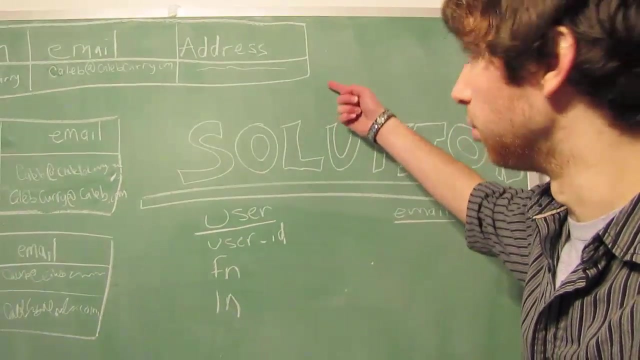 Then we're also going to have an email table. So the solution is to break off the problem column. You can see in this example the email is the thing causing the problem- The address that we had earlier. that's fixable. If it's a problem in the column, we could just break. 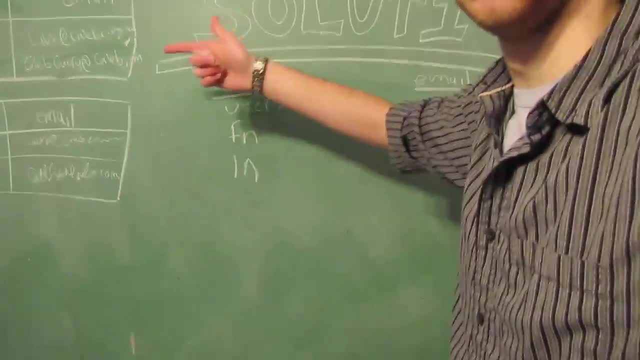 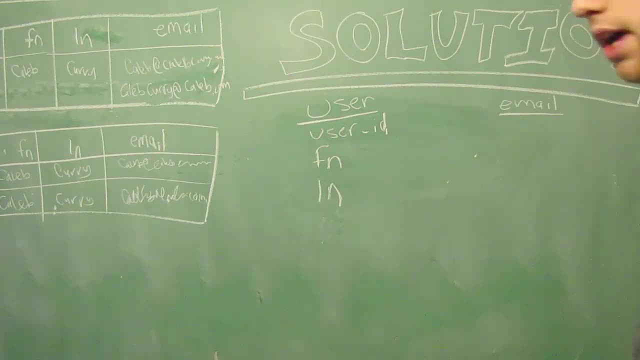 that up into multiple columns, So we wouldn't have to make a new table for that. But since this one, even though the column is correct, it's the values within it that's causing the problem. we would need to create a new table for that. So that's why we have this email table And 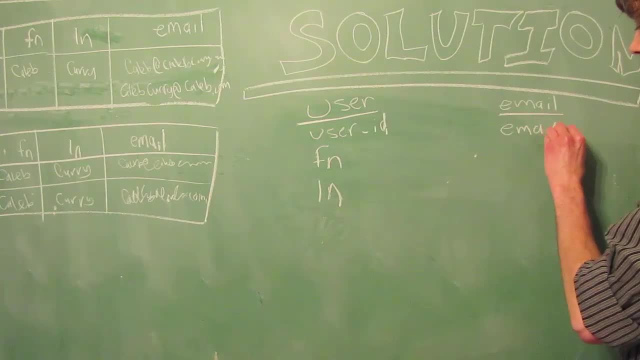 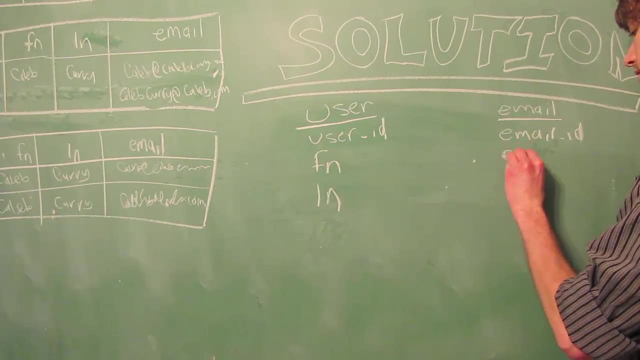 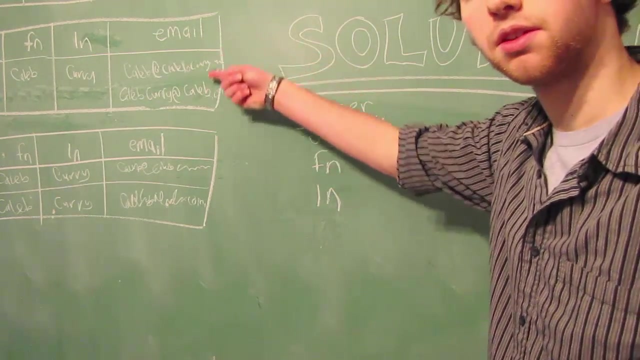 now, within here, we're going to have an email ID, And then we're going to have an email, which is going to be the actual email address, which, in this case, would be these, And then we're going to have a: 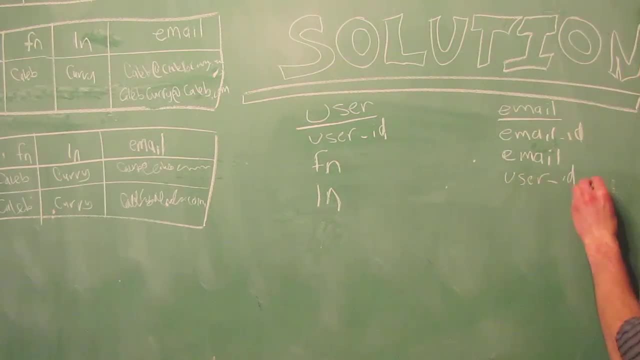 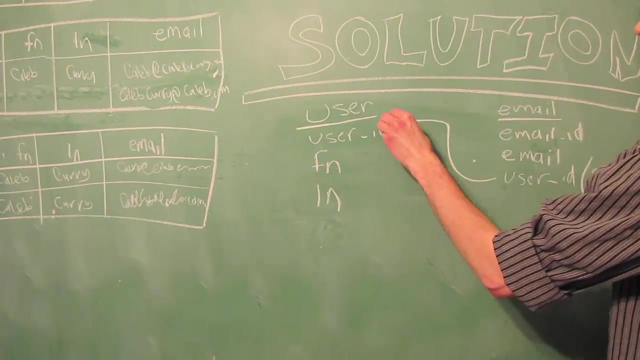 Now, this is going to be a foreign key that references this user ID, The primary key of the 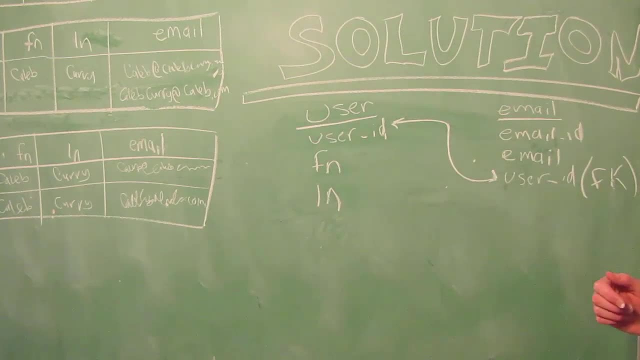 user table. Now, if we wanted to put two individual emails, we could have rows within this email table. Let's spread out the email table and see what it might look like. Here's what the email table might look like. We would have an email table that is a number And that's. 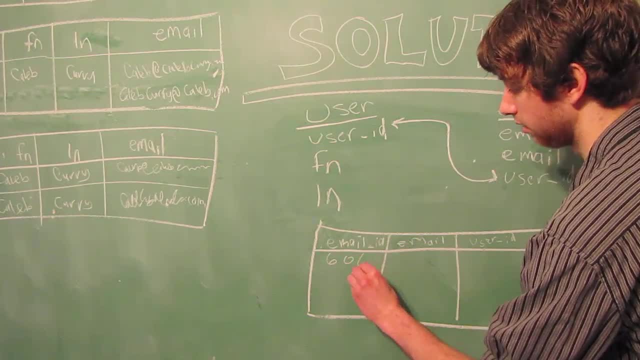 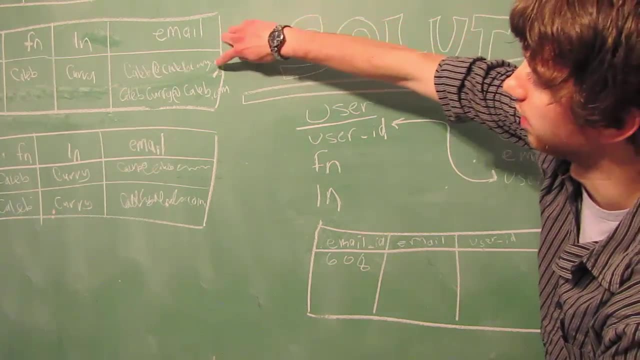 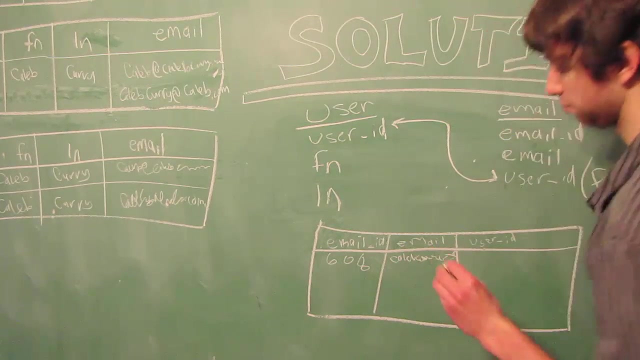 an order ID which is just a randomly generated number for each email- 608 is fine- And then the email that's going to be the actual address of the email. so we could have this- I'll try to make it just as bad as handwriting- Perfect. Then the user ID of who owns that which, in this case, 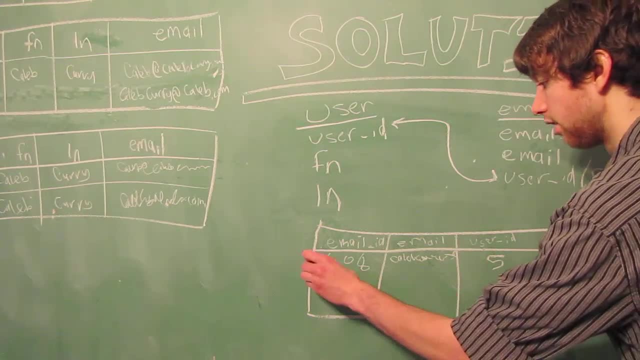 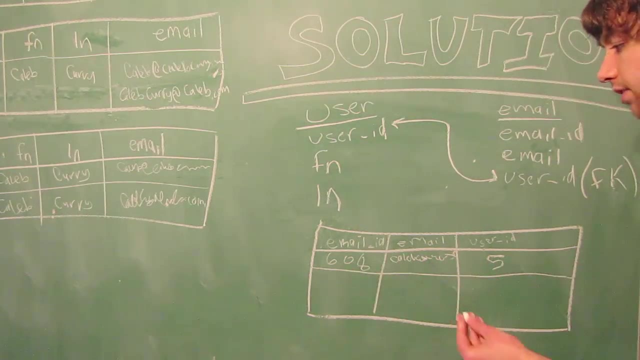 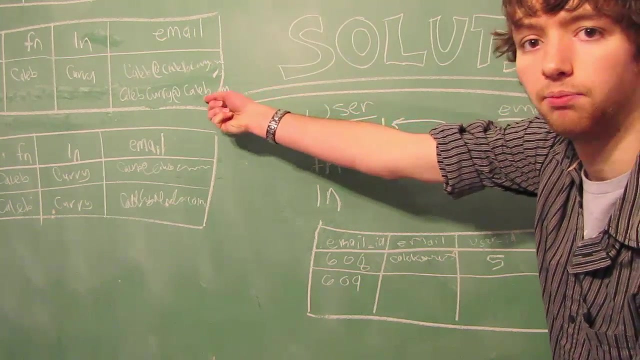 would have been five, because 5 was the ID that was used for this user. This would be our first row. Then we could have another row and it'd be a new email. so we'd have a new email ID. It'd be a different email. We would use this one this time And I'm going to make that beautiful.